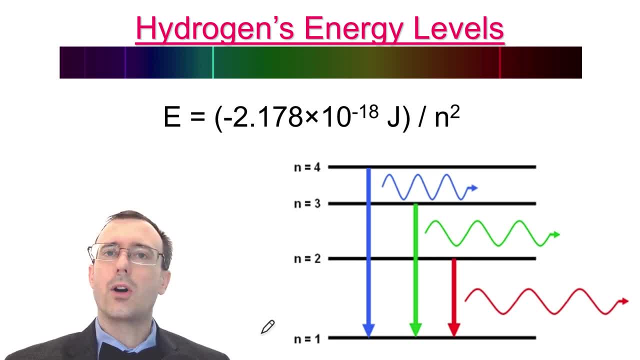 look at this in more detail to understand not only hydrogen but all the atoms, and we can solve for not only the energy level but actually describe and graph those energy levels and see what they look like. That's going to tell us a lot. 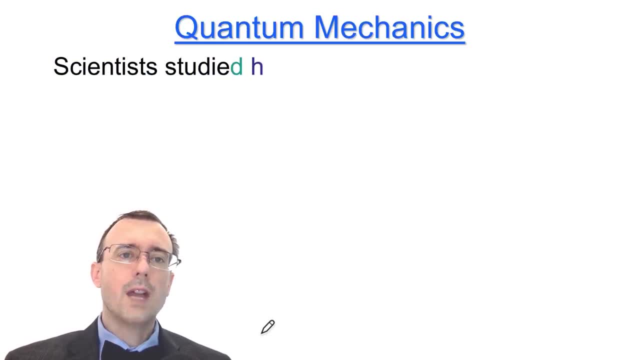 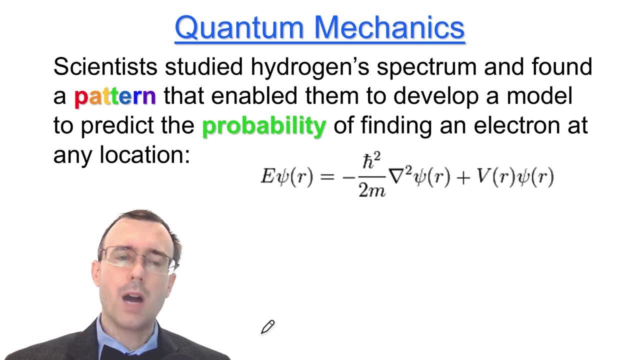 about what the electrons are doing inside the atom. Now scientists studied hydrogen spectrum and found a pattern which we've already talked about, and that pattern enabled them to develop a model to predict the probability of finding an electron at any location. And this equation right. 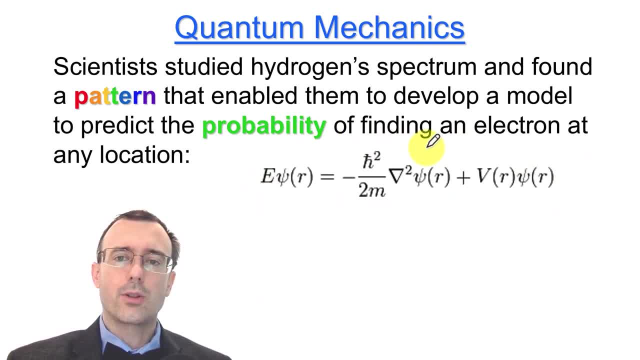 here is known as the Schrodinger equation, right? So the Schrodinger equation is a very, very simple equation to think of in order to assume possible 부탁, For example, as Schrodinger someplace has to have a potential, And you can do this on experiment. Or, for example, 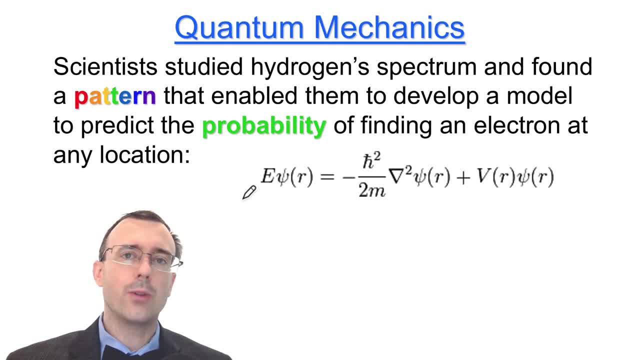 you can do this as aše BO FiST And from there you can do a reaction And to compute a reaction. lookingreso, the acting site of the radiation of places, is a part of the reduction of the energy levels that we have already solved in this class rapidly, then it's already been solved. 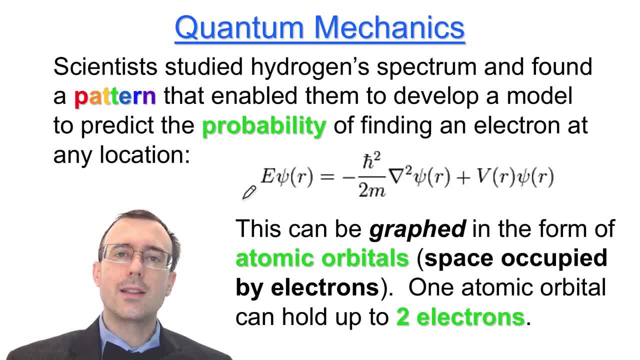 for us, And very nicely, the solutions to this equation have been graphed And those graphs are things that we can look at and describe the patterns of how the different solutions look, the probability of where you're going to find those electrons And because one atomic orbital 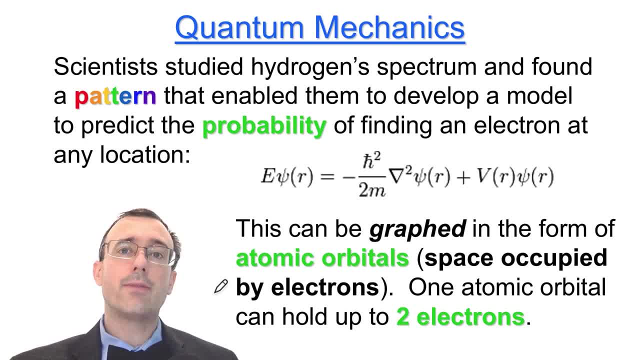 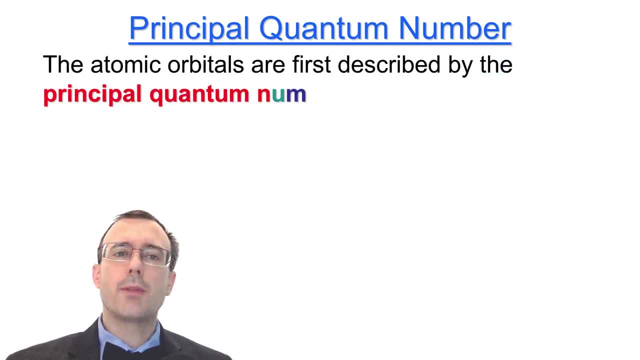 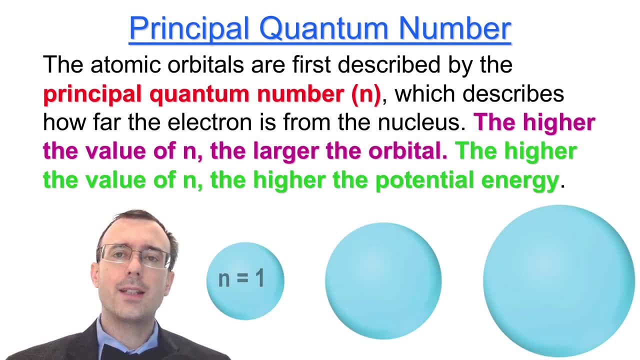 can hold only two electrons. that means most atoms have a lot of different atomic orbitals that have electrons in them. The atomic orbitals are first described by the principal quantum number, n, which describes how far the electron is from the nucleus. So basically, n tells you. 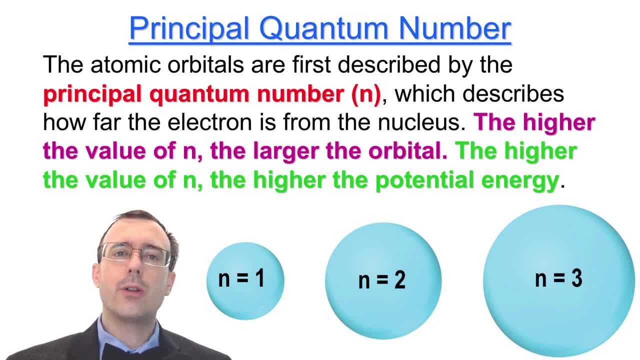 how big the atomic orbital is. The higher the value of n, the larger the orbital. So if we look down here at these three pictures we have here, n equals 1, n equals 2,, n equals 3.. You can see, in terms of those pictures, the bigger the value of n, the bigger the atomic orbital and 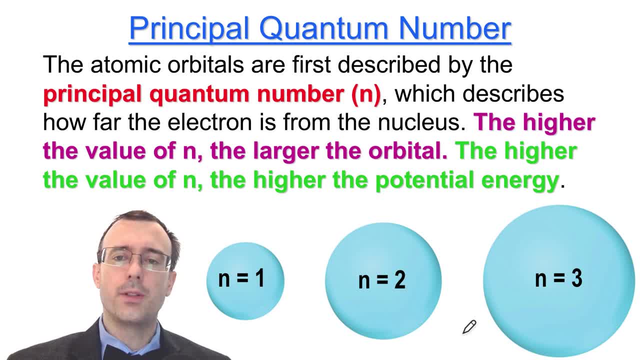 the further on average the electron is from the nucleus. In addition to that, you can also say that the higher the value of n, the higher the potential energy of the electron in the nucleus. So if you look down here at these three pictures, you can see that the higher the 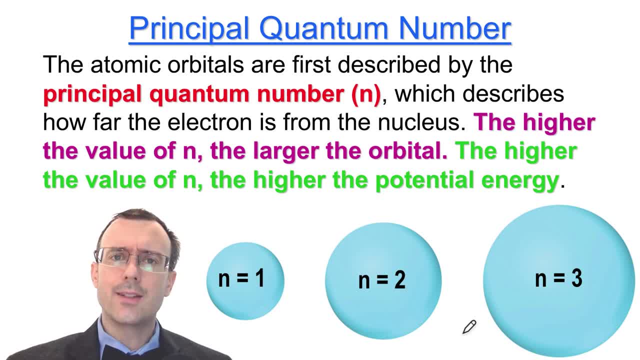 value of n, the higher the potential energy of the electron in the atomic orbital. Now, why is that? The reason for that is that electrons are negative and they want to be close to the positively charged nucleus. So the closer they are, the lower their potential energy. And remember electrons. 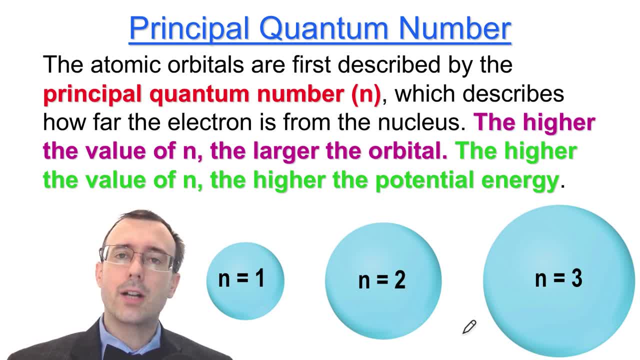 want to go down in potential energy. So as you get bigger and bigger atomic orbitals, their potential energy will increase as they go further away from the nucleus. And remember, they want to be close to the nucleus. Now, we're going to get into the details of this more later, but I want you to 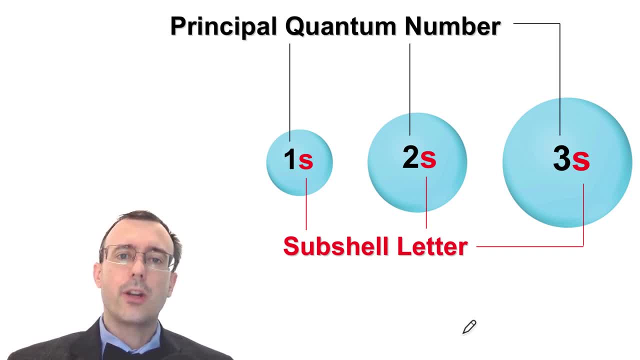 become familiar with how we label the nucleus. So let's get started. So let's start with the nucleus. So now we're gonna label the different atomic orbitals. They are all labeled with a number and a letter. The number that's in front is what we've already talked about. That's the. 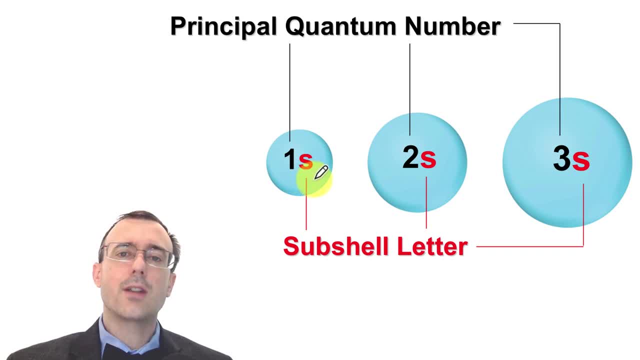 principal quantum number, And the letter that comes after it is the subshell letter, which we're about to talk about. Okay, and so every different atomic orbital can be labeled with both a number and a letter. So this is 1s, 2s, 3s And, as you can see, each of these has all exactly the same. 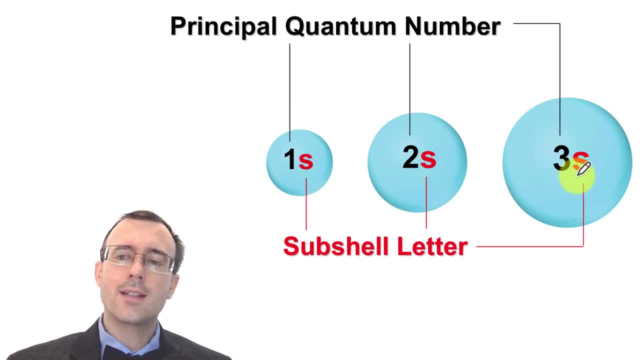 shape, which is why the subshell letter is all the same. right, These are all s subshells, but their principal quantum numbers vary. This is 1,, 2, and 3,, which is why their size is different: n equals 3 is bigger than n equals 2,, which is bigger than n equals 1.. 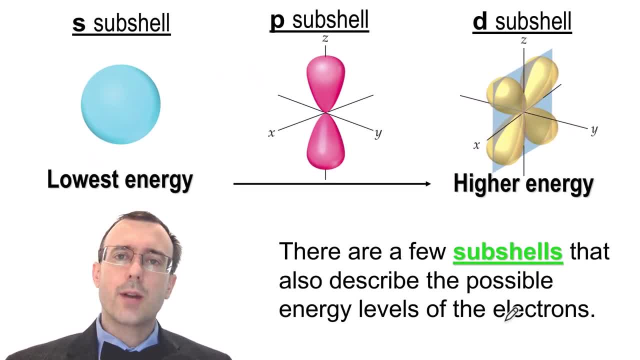 So what about these subshell letters? The principal quantum number describes the size and subshell describes the shape. So we have three different shapes. We actually have a lot more different shapes than that, but I'm first going to just describe three different shapes. 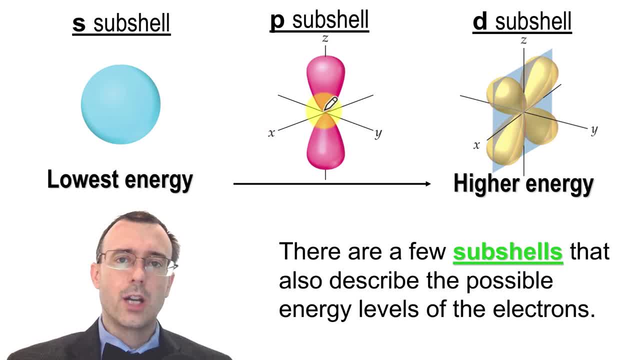 We have the s subshell, which is spherical in nature. You have the p subshell which has got this figure 8 or dumbbell type shape to it, And then you have a d subshell which has this clover leaf type shape to it. And these are not the only different possible shapes. There are more and more. 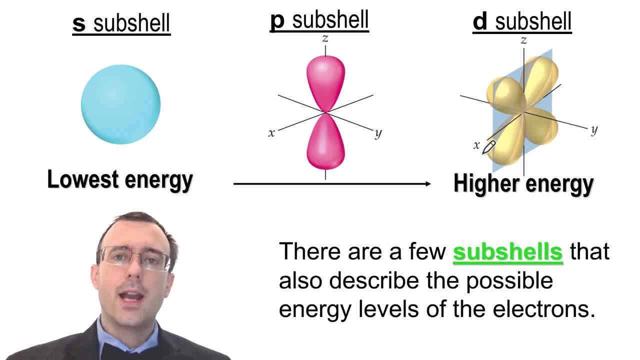 shapes that are also available, but we can already see a bit of a pattern. As you increase the subshell letter, you're going to get a more and more complex shape. So it starts off as s, p, d and then it goes to f, g, h. These subshells not only tell you about the shape. 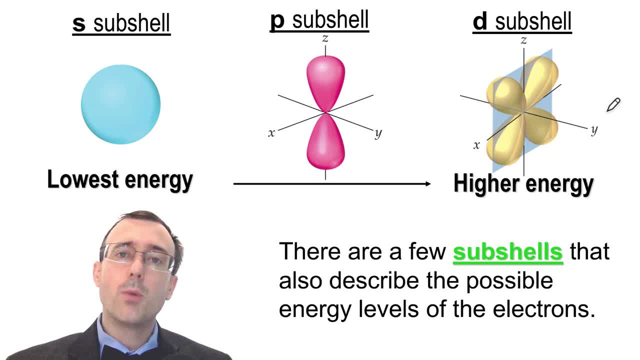 but they also describe the energy as well. The principal quantum number is more important for describing the energy, but these also affect the energy. So the s subshell, which is the simplest and spherical subshell, is the lowest in energy As these shapes get more and more complex. 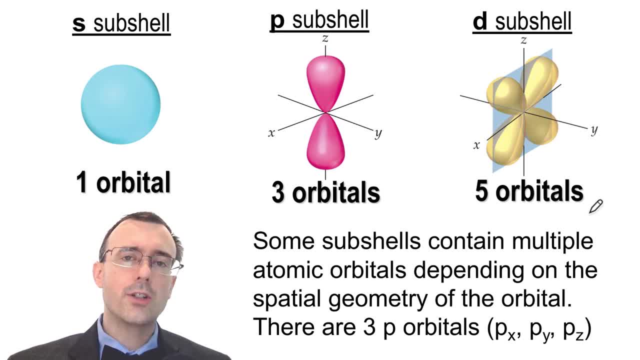 their energy is going to increase. In addition to describing the energy and the shape, these subshells are going to be more and more complex. They're going to be more and more also have a different number of orbitals that are in them. The s subshell has only one orbital. 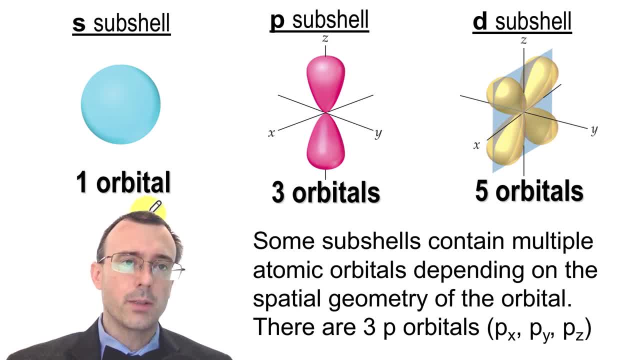 There's not more than one s subshell. So for every principal quantum number there is an s subshell, and each s subshell has only one orbital. The p subshells have three orbitals for each subshell, The d subshells have five orbitals, etc. etc. And we can see a pattern here: One, three, five. 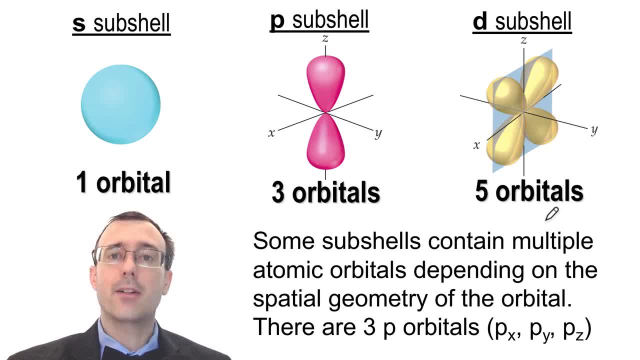 How does that pattern continue? Seven, nine, etc. These are all the odd numbers. So if you were to predict how many orbitals are in the f subshell, well you know that f comes after d. so we know there are seven orbitals in the f subshell. 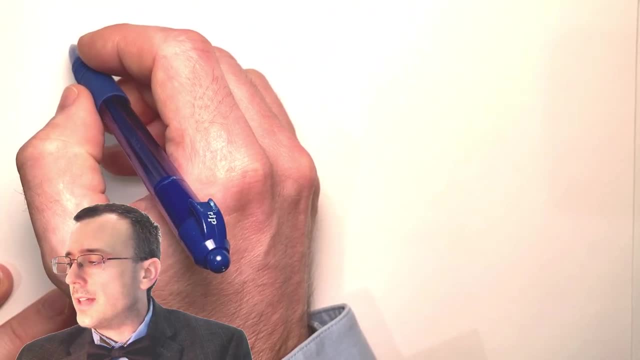 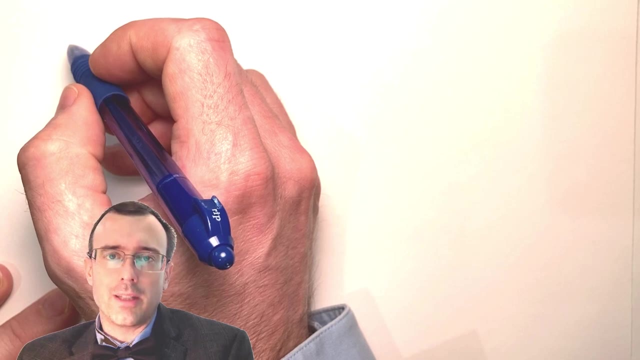 All right. so I showed you guys some pictures of the s, p and d subshells, but I want to go ahead and show you how I draw them, Because if you try to draw them exactly the way a computer draws them, it's going to be a little bit difficult. Now the s is fairly simple, All right. 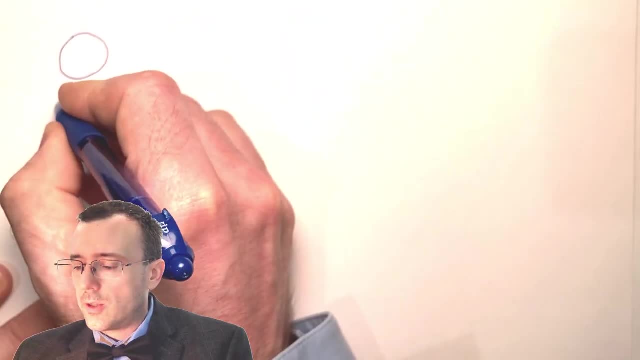 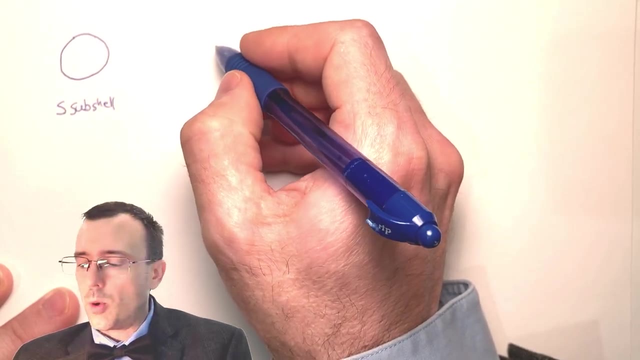 I'm going to draw a circle for an s subshell. All right, so this is going to be our s subshell. All right. now the p subshell we're going to draw more or less like an eight, So you can draw it like: 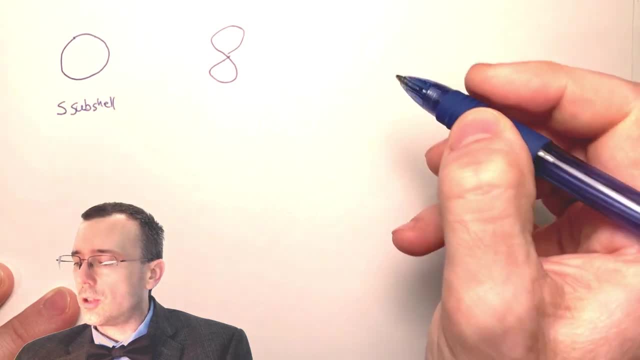 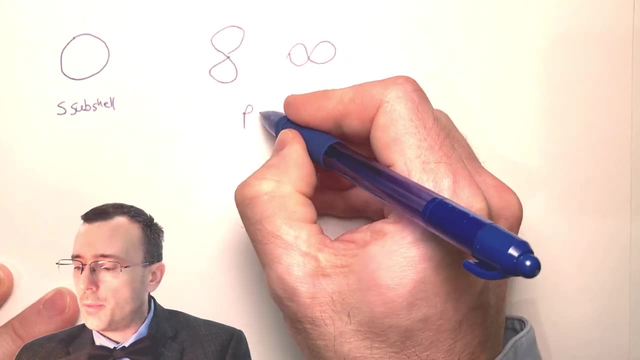 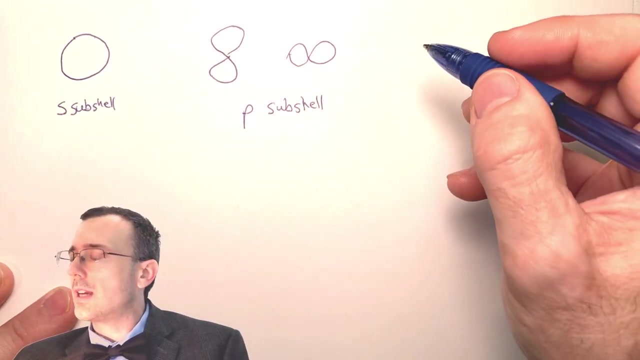 this, so you have kind of an eight look to it. Or you could draw it more like an infinity symbol, if that makes you happy. Right? so this is going to be a p subshell. Okay, now the d subshell. we're going to write like a cloverleaf, and you can write it like this at an angle: 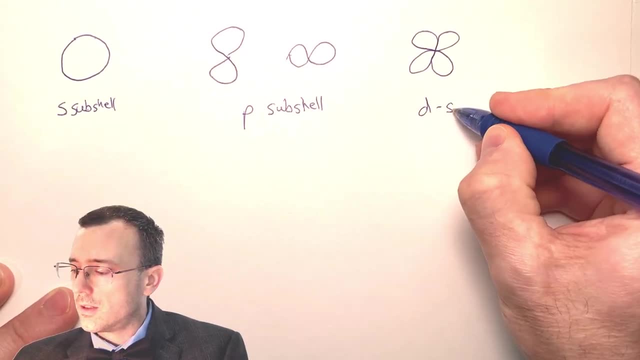 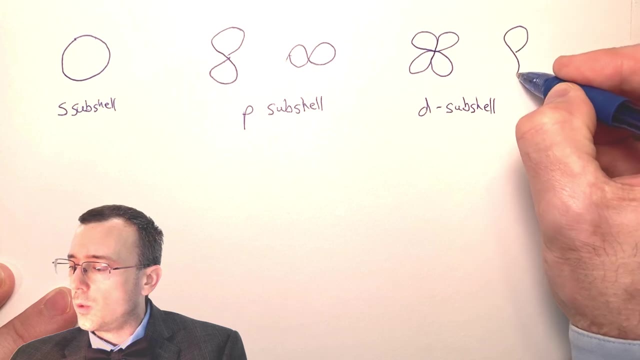 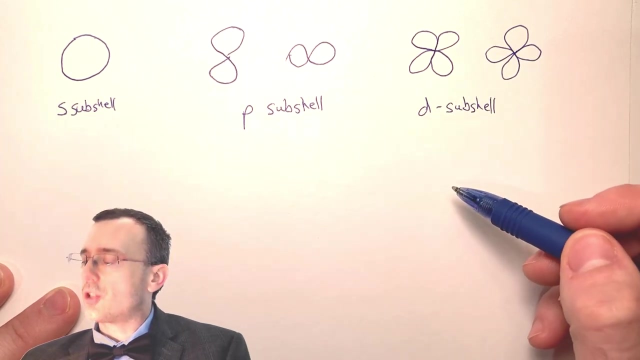 There's your d subshell, Or you can write it with the cloverleaf like this, with an eight first and then your infinity symbol, horizontal. And there's one other shape for the d subshell and I'd like you to learn. 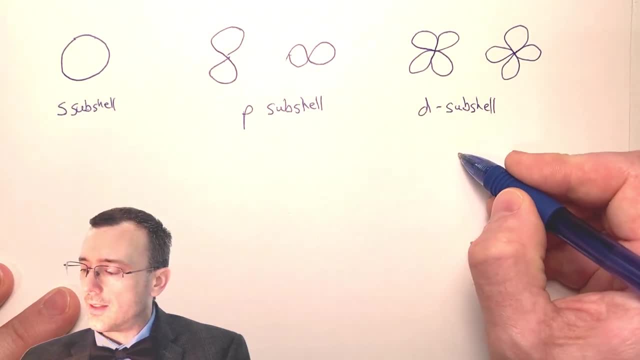 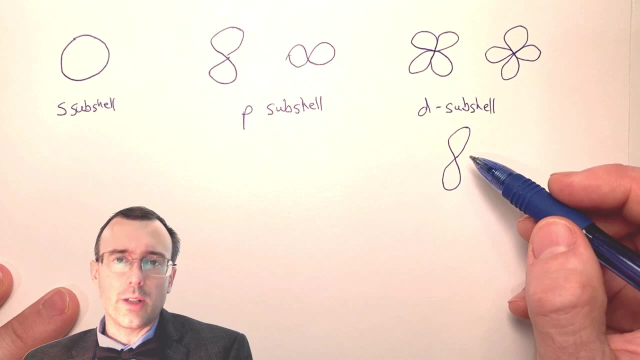 it. So the other shape for the d subshell is this: So first you're going to draw an eight like this, but it's not an eight all by itself. You need to also put a donut around the eight and it looks. 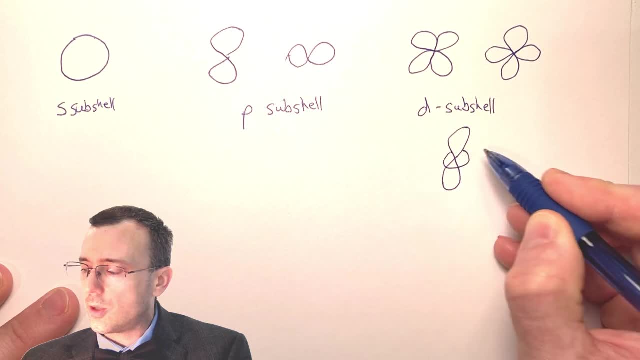 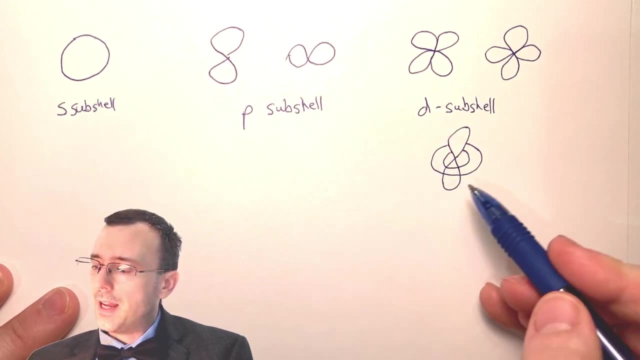 like this. It's more or less like an inner tube around the eight. So you go around like that and then you put another ring around that to kind of give it an inner tube-like look. And if you pencil you could also erase here and here to give it a better look, Or you can maybe predict. 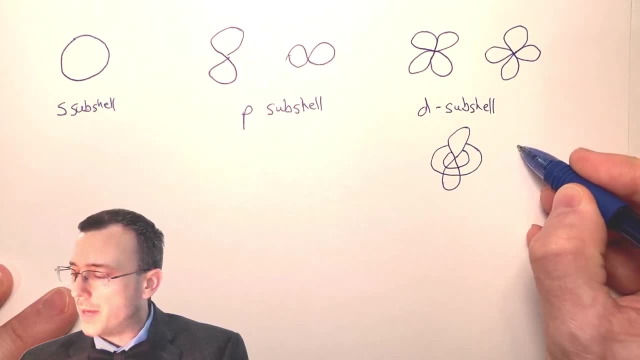 that ahead of time. So it's kind of It's kind of hard to do with a pen, but it's going to be more like this, And so we can draw our first inner tube and then our second ring like this, and you got something like that. So there are your. 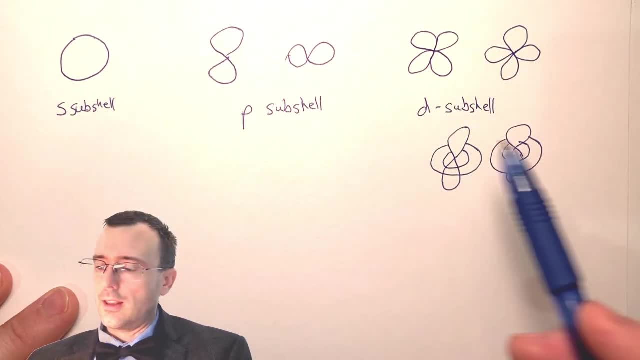 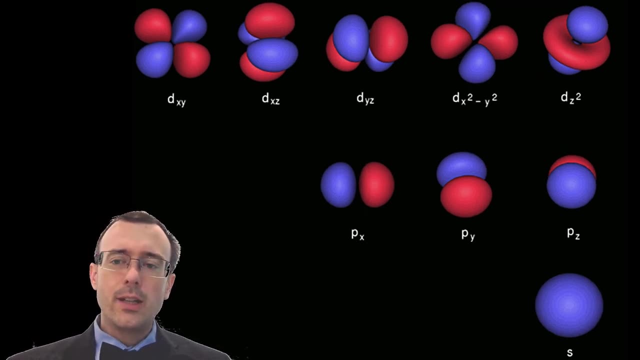 different shapes that you can use for your d subshells. There are your p subshells, your s subshell. Have fun with it. Now. here's a look at All of the different atomic orbitals for the s, p and d subshells. So we see here at the bottom. 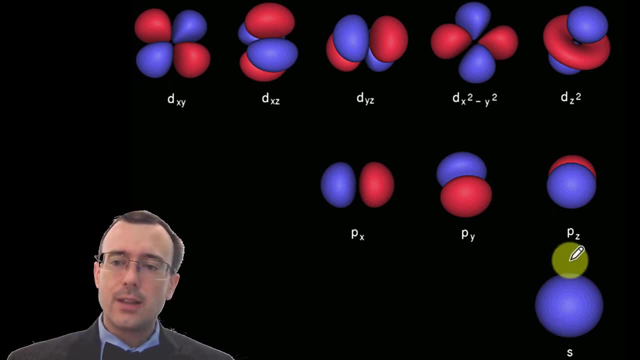 right, this is an s right, It's just a sphere. Now the p subshells can be oriented multiple different ways in space. So we have one like this, one like this one like this And the d subshells. we have five different orbitals for one d subshell And we notice that they are oriented. 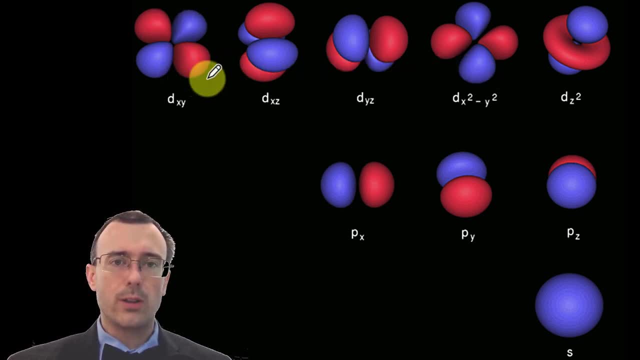 different ways in space. right, You can have this cloverleaf oriented different ways in space and you also have this extra shape for the d orbitals, So very cool. These are graphical representations that were done by a computer, but we now have microscopes that can actually see. 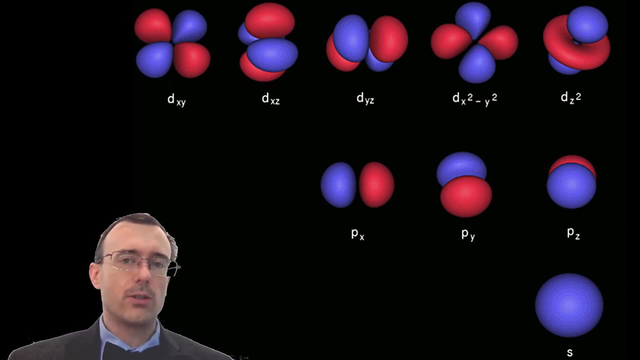 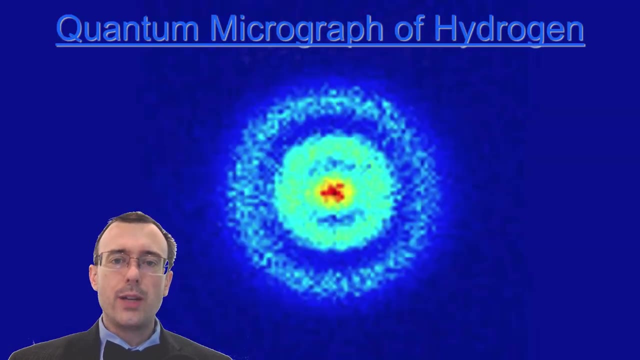 into the atom. This is so cool. This was only invented a few years ago. We have pictures of different atoms, and this is known as the quantum microscope. So this is a picture of a hydrogen atom, And what you're seeing inside of the hydrogen atom are the d orbitals. So this is a picture of a. 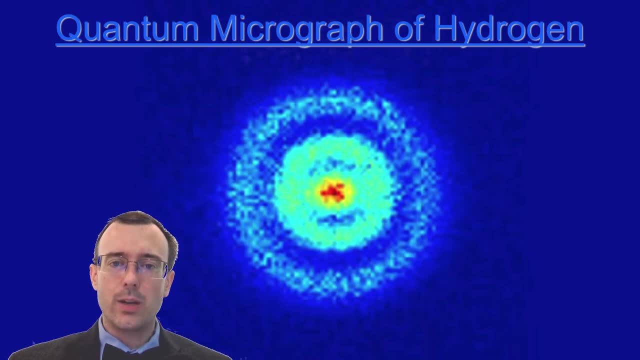 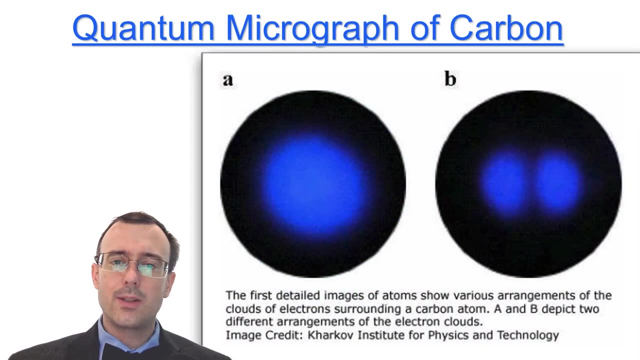 different atomic orbitals. Now I don't know exactly which one's which, but you can see the different atomic orbitals within the hydrogen atom. This is a picture of a carbon atom and you can see clearly that you have an s subshell and a p subshell and you've got different atomic orbitals. 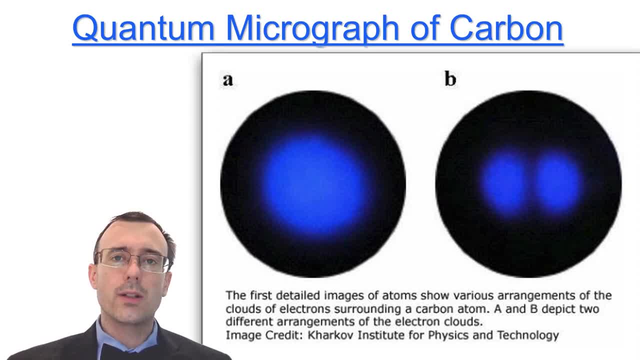 shown there. So super, super cool. These atomic orbitals are not simply just somebody's theory or some kind of mathematical solution or computer simulation, but we can see through the quantum microscope that they're real and they have a real physical thing that we can measure. to show that these 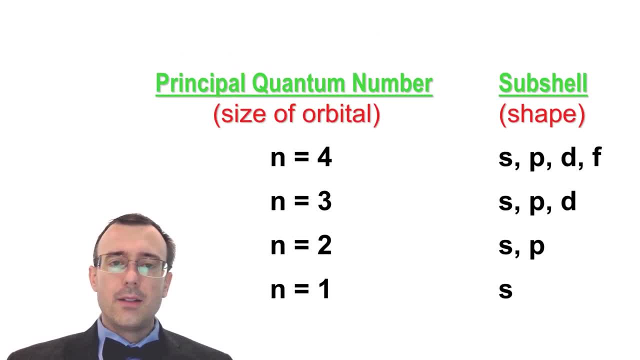 atomic orbitals actually exist. Now, in addition to that, there are a number of different rules and patterns that help us to understand how the electrons can go into the atom. Now let's see. First of all, we have the principal quantum number. So a little bit of review here. The principal: 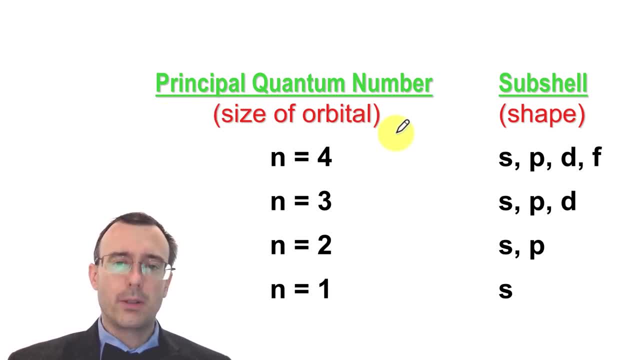 quantum number tells us about the size of the orbital. The bigger the number, the bigger the size. And then you have the subshells, which tell you about the shape. The higher and higher this subshell, the more complex shape you have. Now, in addition to that- not all of the subshells- 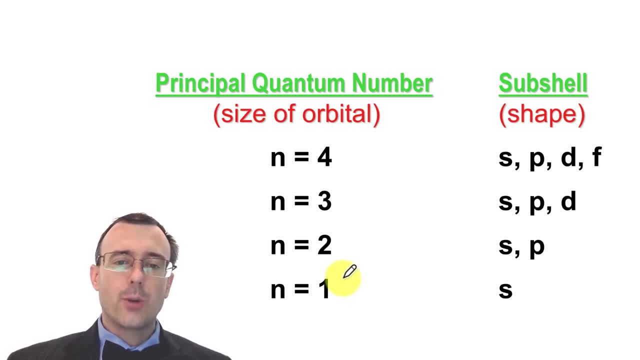 exist for every principal quantum number. okay, So for a principal quantum number, or energy level one, there's only the s subshell and that's it. There is no one p or one d or one f, There's only a one s, There's only the s subshell, for n equals one As you go up in principal quantum number, so up to: 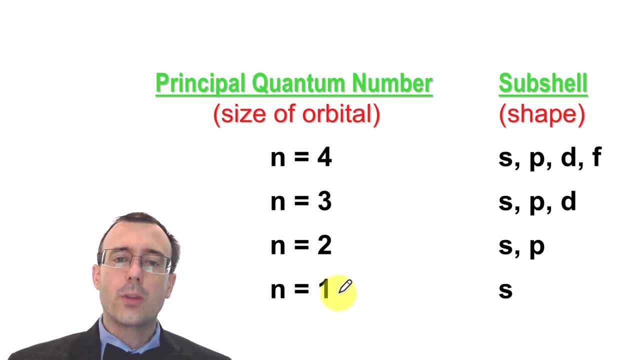 you. you now have an additional subshell. So the principal quantum number not only tells you the size but it also tells you the number of subshells. So for n equals four, you have four subshells. For n equals five. you have five subshells, So for n equals five. you can imagine that would have s, p, d, f and g. 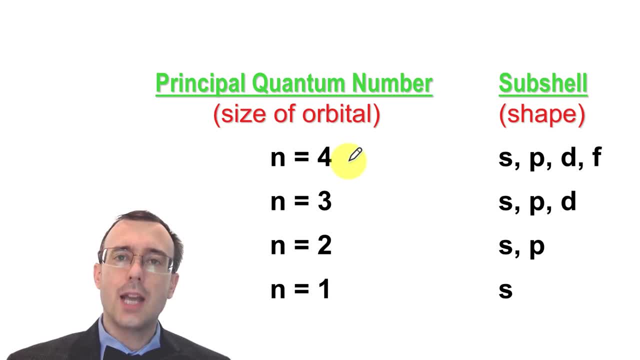 For n equals six. you're going to have s, p, d, f, g and h. So each time you go up in principal quantum number you're going to add an extra subshell. The principal quantum number tells you the number of subshells in it. Now some orbitals. 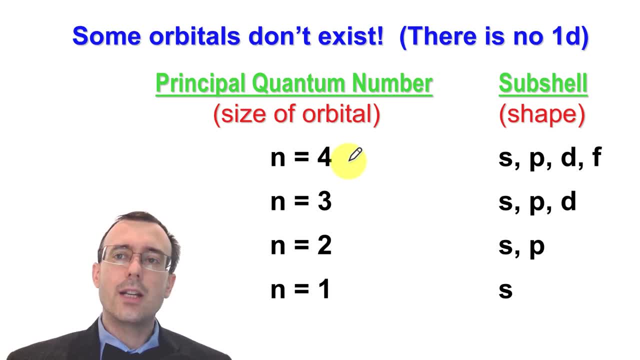 simply don't exist and we have to understand this. So there is no one d. n equals one, has only one s. There's no one p. There's no one d, There's no one f, etc. For n equals two, there's only two s.